Robot arms are being used extensively for various industrial applications such as pick and place, welding, painting, etc. What if you want a robot arm to do a paint job, but it results in something like this? This shows that how important it is to operate the robot manipulators safely, especially when the robot is working collaboratively with humans. 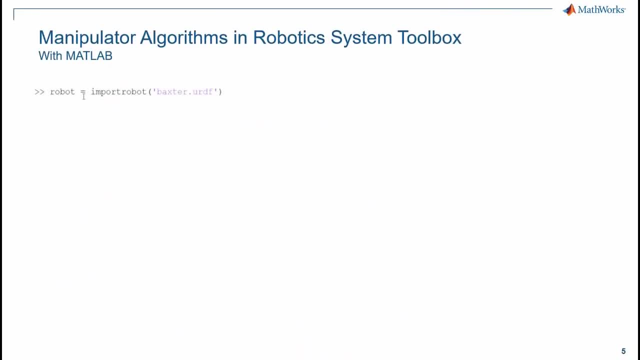 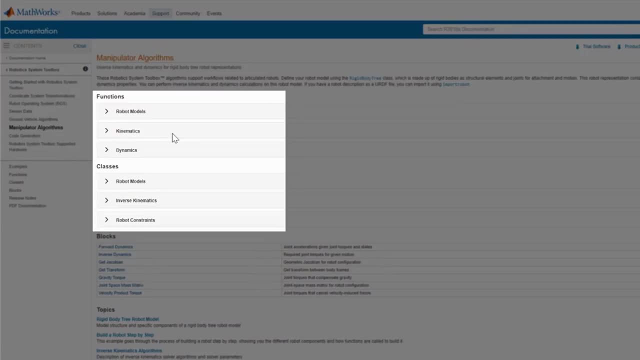 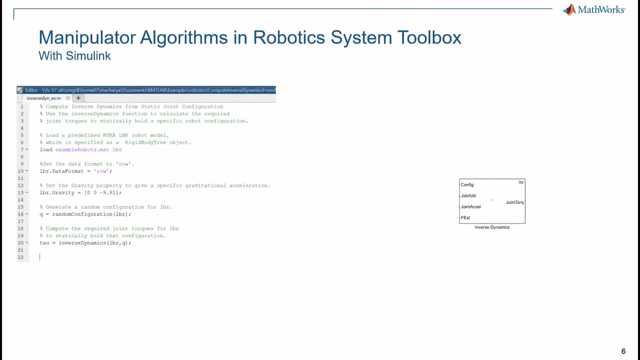 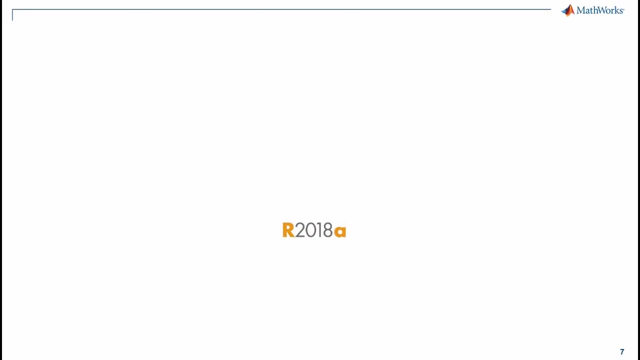 With manipulator algorithms in Robotic System Toolbox, you can write code in MATLAB to define a model of an articulated robot, and you can use the inbuilt classes and functions to perform inverse kinematics and dynamics calculations on this model. Furthermore, using model-based design, you can implement complex algorithms for robot manipulators in an easier and time-efficient way. In the 2018a release, Robotic System Toolbox provides several useful blocks for manipulator algorithms in the Robotic System Toolbox. 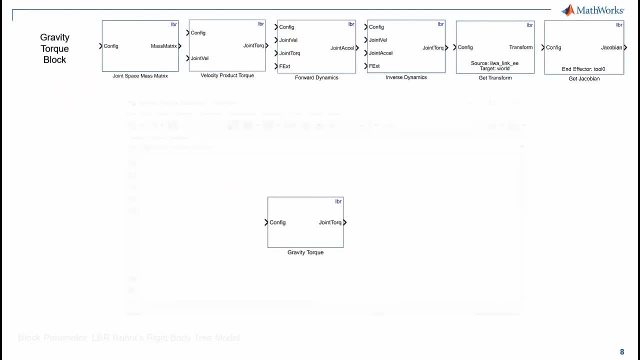 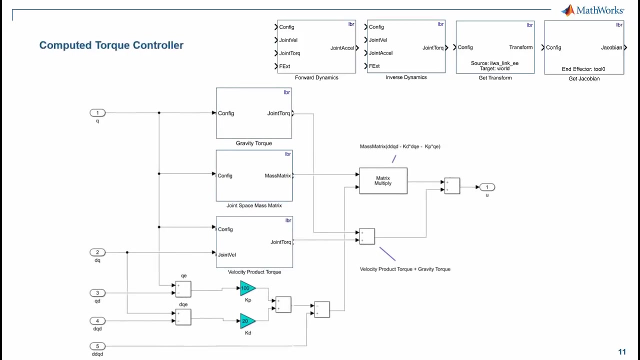 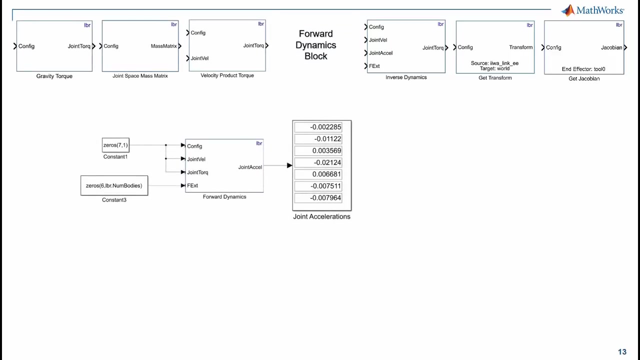 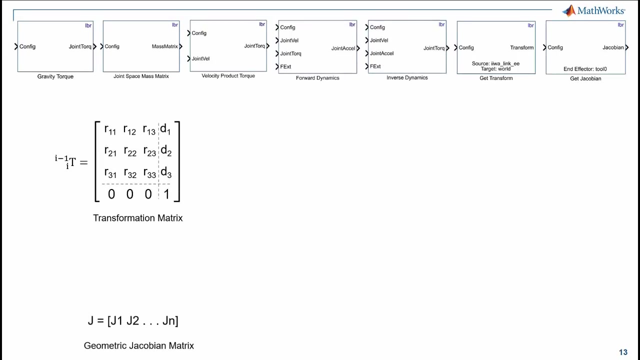 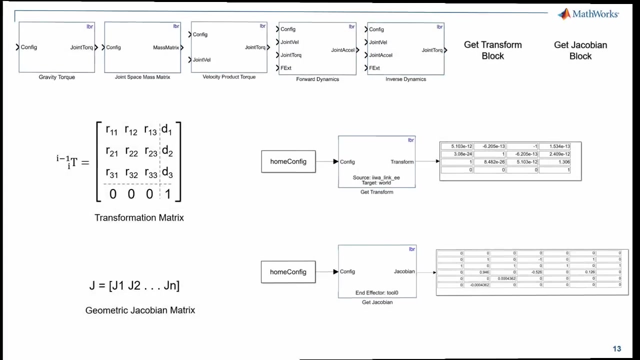 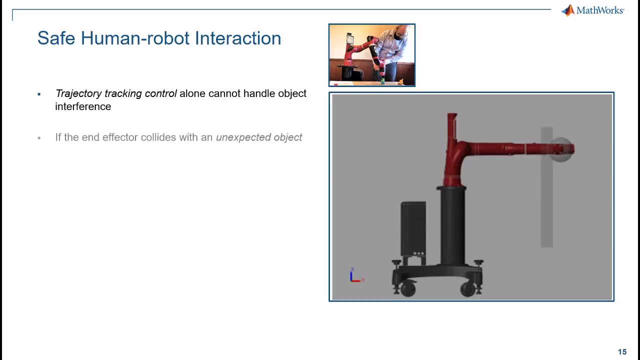 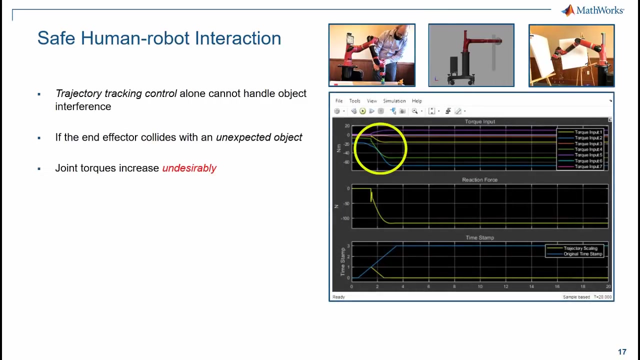 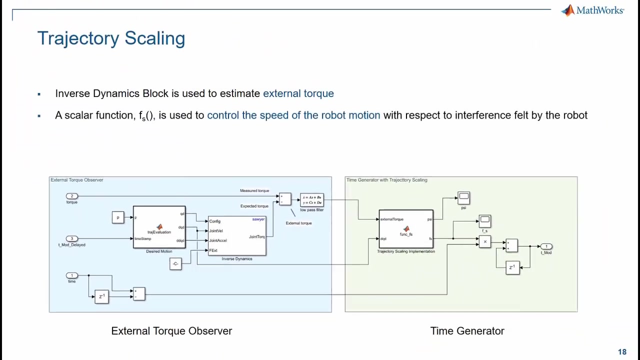 Let's talk about the modules we're going to discuss now – SOLO Mushroom Color, simple energy stimulation,asia The first module is called Stud. to obtain joint accelerations by giving applied talks and states as inputs or even better inverse dynamics block to calculate joint talks and maintain a specified robot state by giving joint accelerations as input for performing calculations like robot body transformations and obtaining the geometric Jacobian you can use get transform and get Jacobian block now let's go back to the concern of safe human-robot interaction in trajectory tracking control without the safety feature when the robot collides with an unexpected object like the styrofoam sheet there is an undesired increase in the joint talks and that causes the damage you can use the inverse dynamics block with additional components to implement trajectory scaling algorithm which helps to 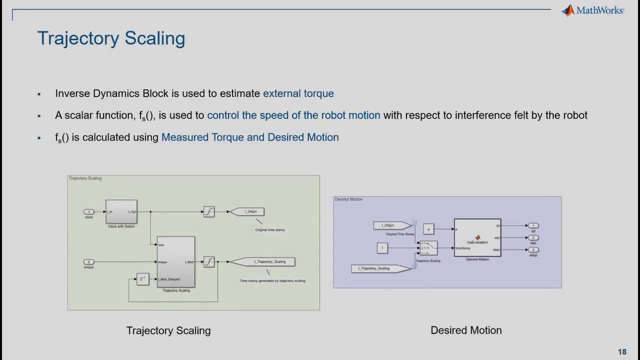 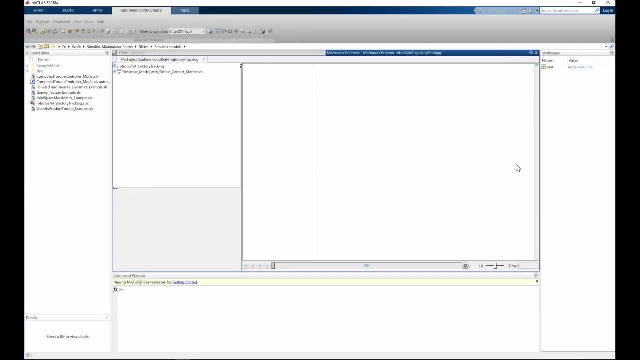 control the speed of robot motion and regulate torque values robotic system toolbox provides an inbuilt model that uses these blocks to simulate safe trajectory tracking control on a rethink Sawyer robot arm the models we saw in the previous video are the same as in the previous video the